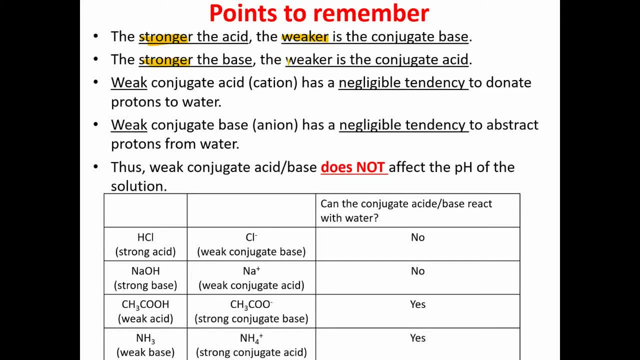 conjugate base. Same score for base. Stronger base, weaker conjugate acid. So weak conjugate acid and weak conjugate base. they have negligible tendency to be acidic For acid conjugate. for weak conjugate acid it is negligible tendency to donate. 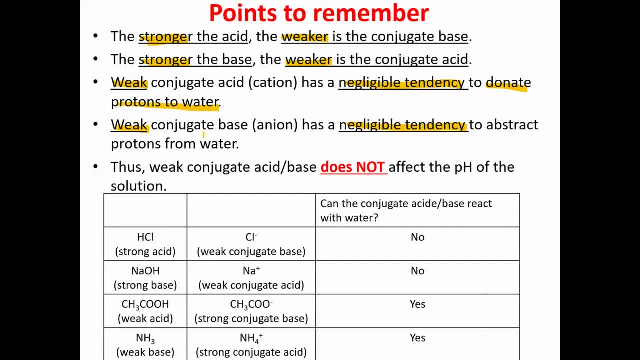 protons to water Means. it cannot donate proton to water. Weak conjugate base is the same. It cannot accept proton from water. Thus very important here. weak conjugate acid or base does not affect the pH of the solution. For example, HCl-, NaOH, Hychloric Acid and Sodium Hydroxide, both of 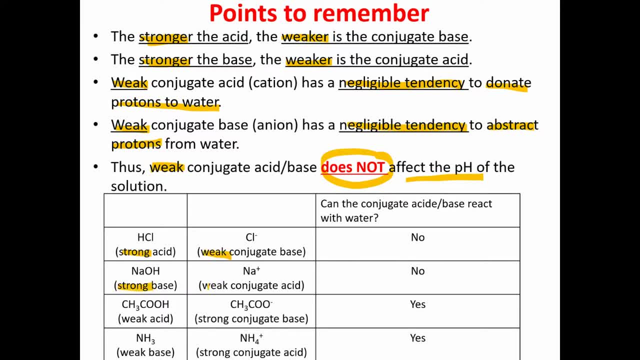 them are strong acid and strong base. Thus the conjugate base and conjugate acid are weak. Therefore, the Katenion and National Ion or the conjugate acid or base will not react with water. However, the weak acid has strong conjugate base. The weak base has strong. 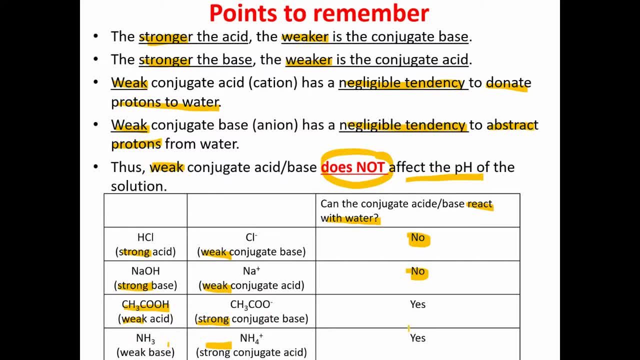 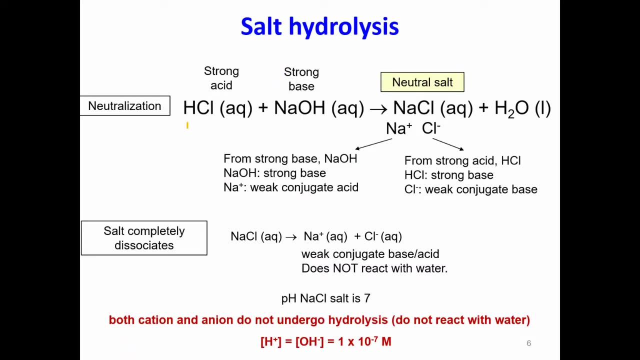 acid. thus the strong conjugate acid or base can react with water and thus it will affect the pH. now let's look at example. okay, when so hydrochloric acid react with sodium hydroxide, strong acid and strong base, we get neutral salt. okay, what when the salt completely dissociate? okay, we didn't, we will get sodium plus. 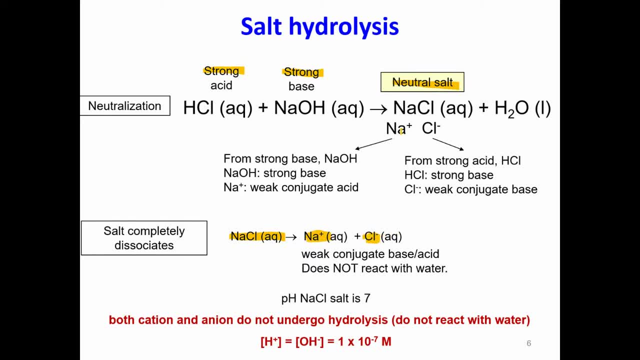 sodium ion and chloride ion. okay, so remember, sodium is come from. sodium. ion comes from strong base, thus is is a weak conjugate acid. then chloride ion comes from strong, strong acid. okay, it's come from strong acid. so, when it comes from strong acid, thus, chloride ion is a weak conjugate base. okay, remember, weak conjugate acid or base. 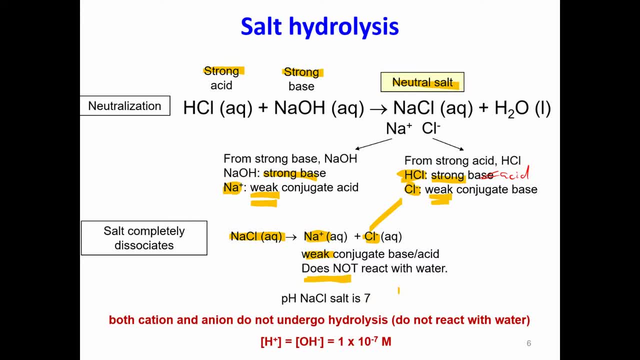 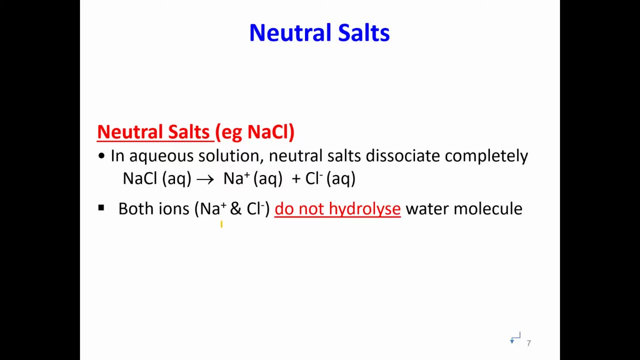 does not react with water. thus it does not affect the pH. therefore it is neutral. so we can say that both cap ion and anion do not undergo hydrolysis. okay, so this one is a summary. in aqueous solution, neutral salts dissociate completely and then both cap ion or anion or the conjugate acid, the 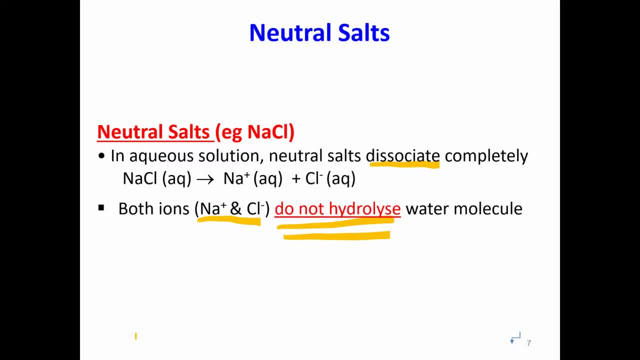 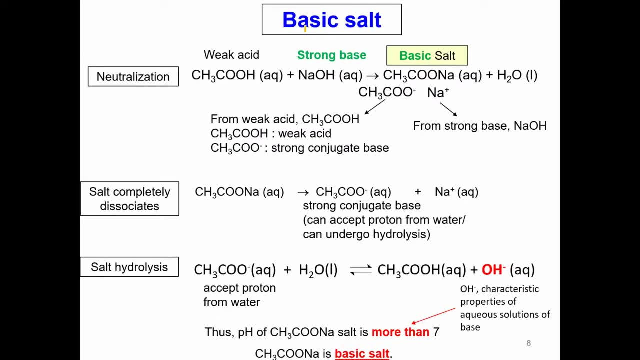 conjugate acid, conjugate base do not hydrolyze water molecule. therefore it is a neutral salt. now next one: we go to basic salt. when weak acid react with strong base, we get basic salt. okay, why now salt completely dissociate? we will get CH3, COO minus and sodium ion. okay, what happens here? 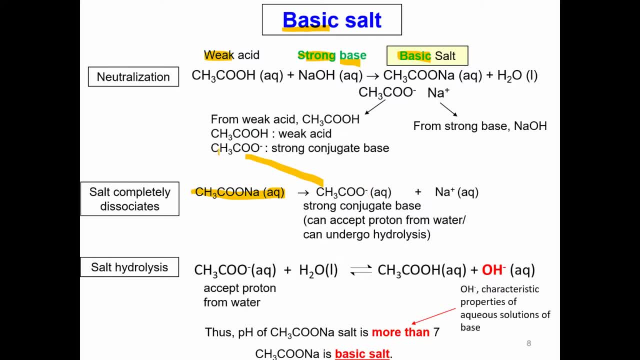 okay, how do we know CH3 COO minus is strong or weak? okay, CH3 COO minus ion comes from weak acid. so weak acid means strong conjugate base. if strong conjugate, then it can accept proton and it can undergo hydrolysis means that it will affect the pH. okay, 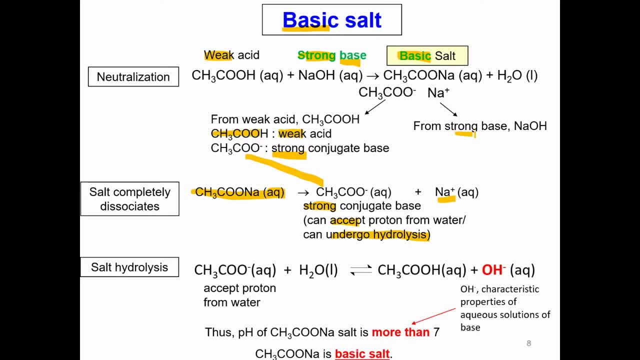 then from here, sodium ion is from strong base. if it's from strong base, that means that it is a weak conjugate acid. weak conjugate acid cannot undergo hydrolysis. thus the pH it will be determined by the CH3 COO minus and CH3 COO minus and CH3 COO minus. 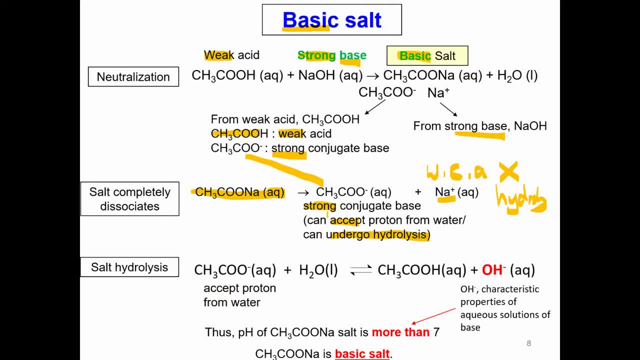 is strong conjugate base. okay. so what happened is CH3 COO minus can accept proton from water and then, after reaction, it will produce OH minus. OH minus is the properties of characteristic properties of aqueous solution of base. okay, because of this, we know that CH3 COO Na is a 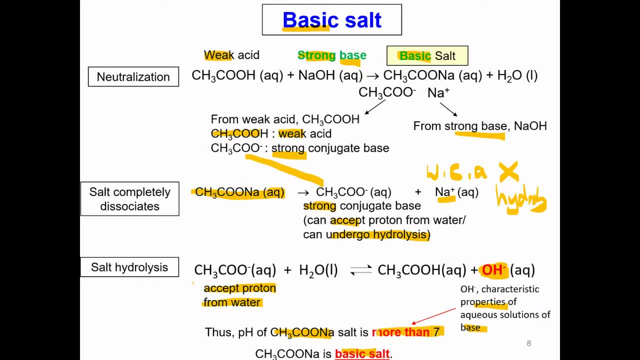 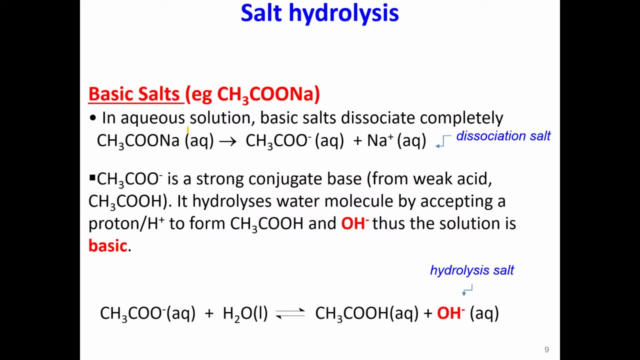 basic salt because we have the pH will be more than 7. okay, so remember, this is a conjugate base. base accept proton, so water will react as acid. okay, in short, we say that in aqueous solution basic salt dissociates completely. then we say that at CH3 COO minus ion is. I must mention that they are strong conjugate. 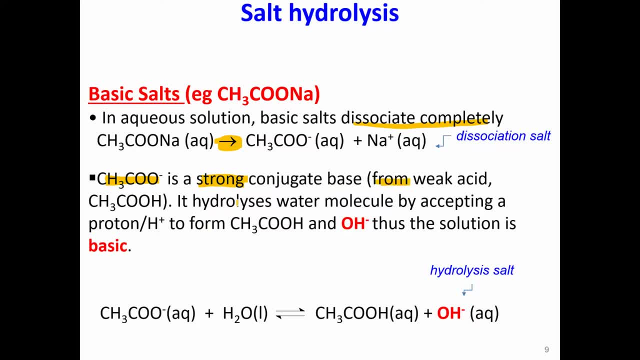 base from where weak acid, Thus the strong conjugate base, can hydrolyze water molecule by accepting a proton to form CH3, COO, H and also OH minus. thus the solution is basic and then you must show the reversible reaction. okay, so remember, you need to show one of the reaction. is this completely dissociation? 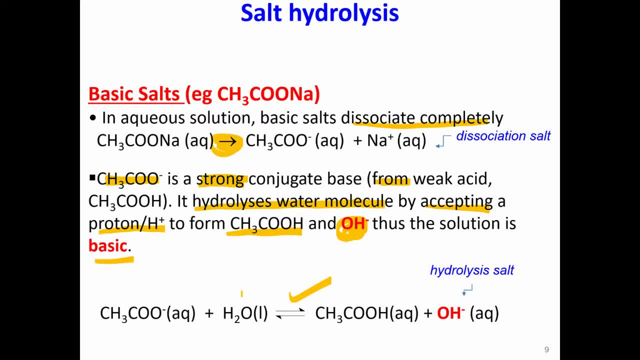 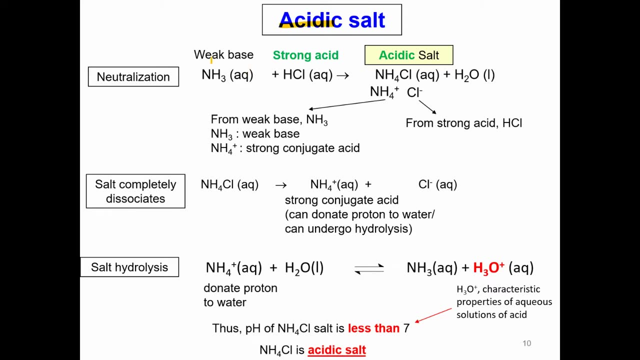 of salt, single arrow. And then when the conjugate base or conjugate acid can hydrolyze the water, you must use reversible arrow, because they are weak, Okay. next one: we go to acidic salt. So when weak base react with strong acid, you get acidic salt, okay. 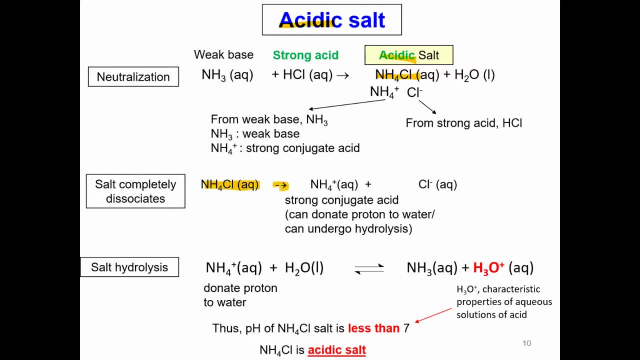 So this salt, ammonium chloride, will completely dissociate. okay. so we know that CL minus comes from strong acid. So if come from strong acid means it is weak conjugate base, it does not hydrolyze, okay. But ammonium ion is a strong conjugate base, a strong conjugate acid, because it comes from 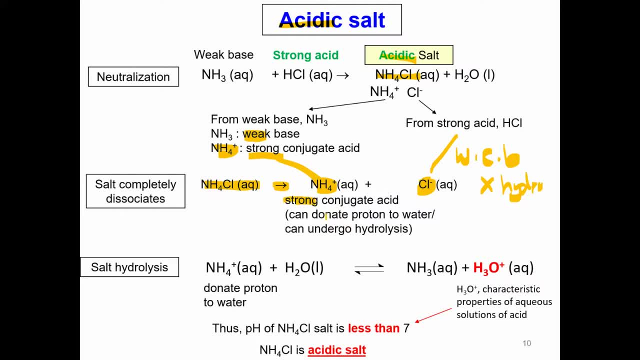 weak base. so strong conjugate acid can donate proton to water, or they can undergo hydrolysis, okay. So here it will donate proton to water, Okay, And then you will get H3O plus. So H3O plus is the characteristic properties of aqueous solution of acid, thus the pH of